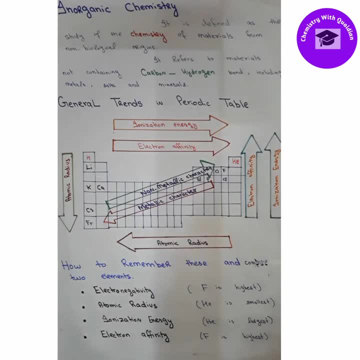 Only that are hydrocarbons, While in inorganic chemistry we study all the elements in the periodic table except hydrogen and carbon. So it refers to materials not containing carbon and hydrogen bonds, including metals, salts and minerals. All the elements except carbon and hydrogen are studied in inorganic chemistry. 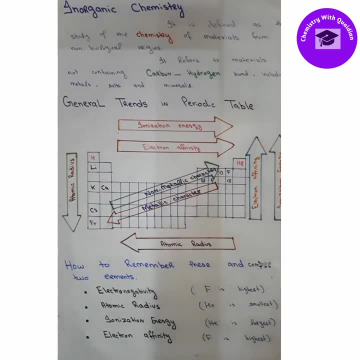 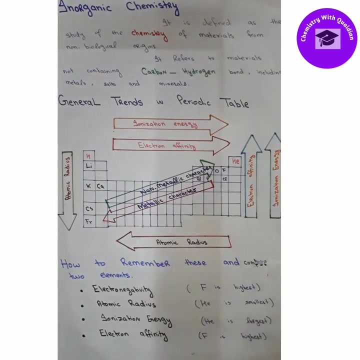 Now let's move to the general trends. in periodic table, The most commonly studied trends are of electronegativity, atomic radius, ionization, energy, electron affinity trends. Now, first we will discuss electronegativity trend. Electronegativity is the force to attract the shared pair of electron toward itself. 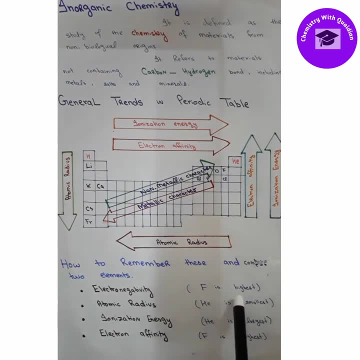 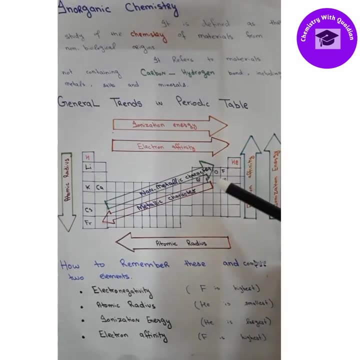 We know that among all the elements, fluorine has the highest electronegativity. It belongs to group 7a here, the halogen family. So those elements that are close to fluorine have high electronegativity. Then those elements that are far from the fluorine, 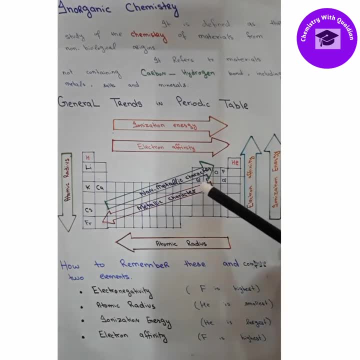 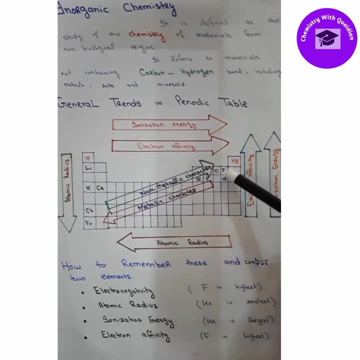 So if we have to compare two elements, like we have to compare aluminum and cesium Among these two elements, aluminum have high electronegativity because it is close to fluorine atom And cesium have low electronegativity because it is far from fluorine atom. 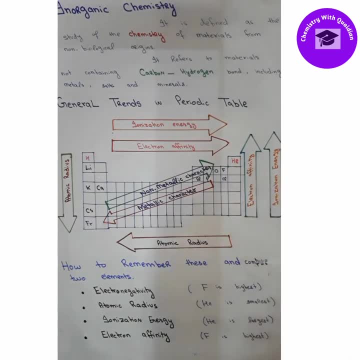 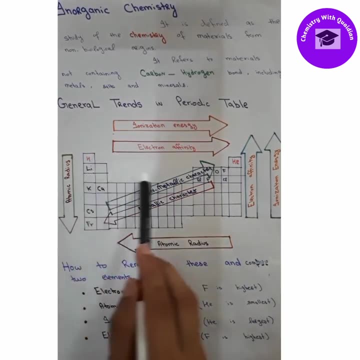 In this way we can generate a trend that electronegativity basically increases from left to right in the periodic table. From Lithium to fluorine, it increases. Now let's move to atomic radius. What is atomic radius? Atomic radius is basically the size of the atom. The size of the atom we know increases when the number of shells in the atom increases And we know that number of shell increases down. the group And number of shell remain constant along the period. So helium is the smallest. Helium is the smallest atomic radius. 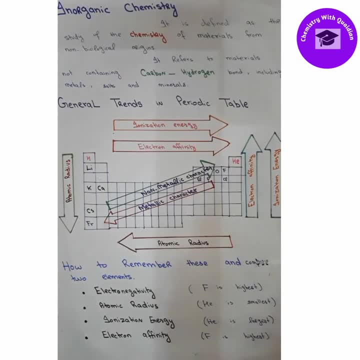 So those elements that are close to helium have small atomic radius, While those which are far from the helium have large atomic radius. For example, we will compare chlorine with the friendship. So chlorine will have small atomic radius, While friendship will have highest atomic radius. 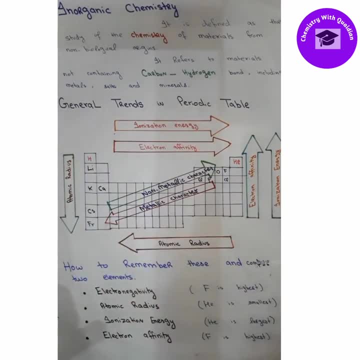 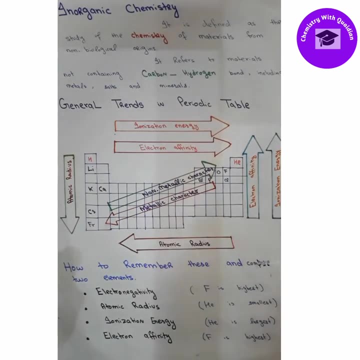 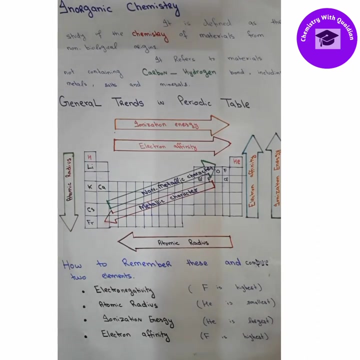 It will have highest atomic radius among all the elements because it lies totally opposite to the helium atom, If we compare all the other elements. Now let's move to ionization energy. Ionization energy is the amount of energy required to remove an electron from the outermost shell. 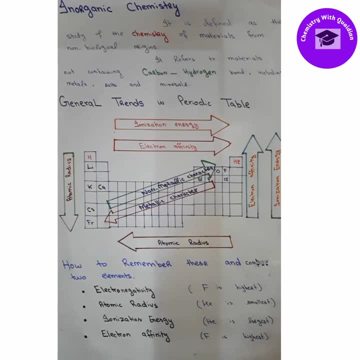 Means those elements that have loosely bound electron will lose their electron easily and their ionization energy will be low. And those atoms which have tightly bonded electron cannot lose their electron easily and their ionization energy will be higher. So we know the noble group metals. 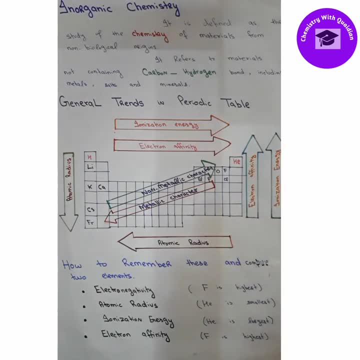 Noble group metals have complete octet. Their electrons are tightly bound So it is very difficult to remove electron from them. So helium has the highest ionization energy. So the elements which are close to helium have high ionization energy. 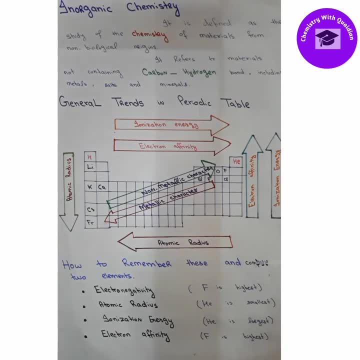 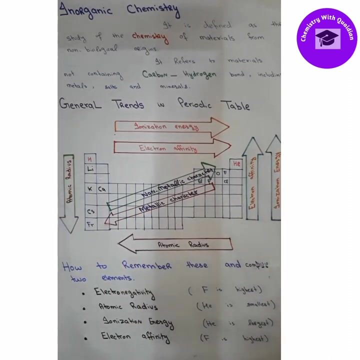 While those far from helium have low ionization energy. Here we compare oxygen with the helium, Here we compare oxygen with the helium, Here we compare oxygen with the helium. Oxygen close to helium will have high ionization energy, And potassium very far from helium will have very low ionization energy. 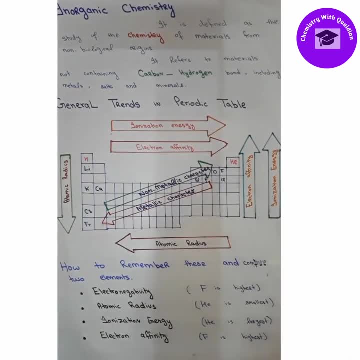 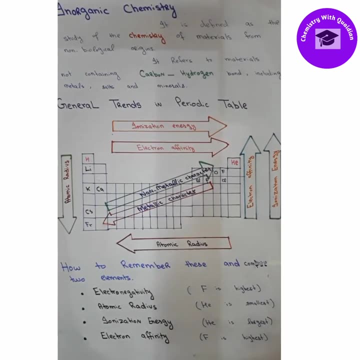 So here the trend is also ionization. energy increases along the period. Now talk about electron affinity. Electron affinity is the energy released when an electron is added to the outermost shell. Now, which elements among the purules do we have? 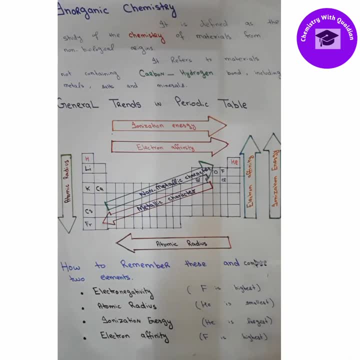 elements among the periodic table are the hungriest for the electron. We all know that these are the halogen family. They have one electron less than the octet, So they want to gain one electron very quickly to stabilize themselves In this way their electron affinity. 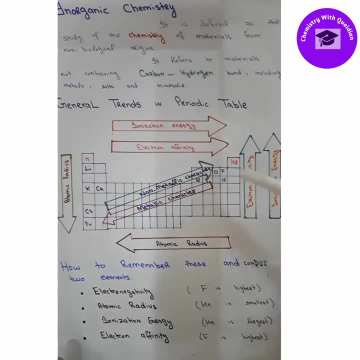 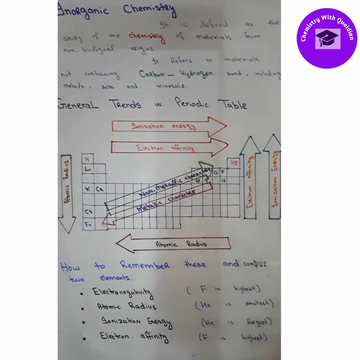 is very high. So fluorine has the highest electron affinity among all the elements. So those elements that lie close to fluorine have high electron affinity, while those far from fluorine have low electron affinity. For example, we have compared now phosphorus and cesium, For example. phosphorus have high electron affinity and cesium have low electron. 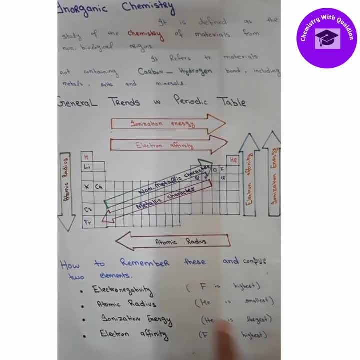 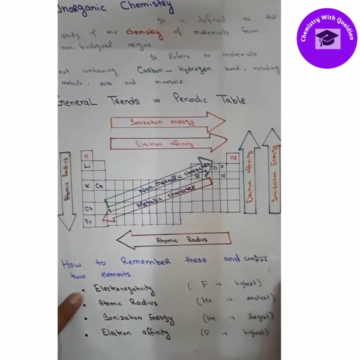 affinity. So the general trends for these are: electronegativity increases from right to left to right in the periodic table. Atomic radius decreases from left to right in the periodic table. So like this—it helps for merchandising- for lithium, calcium, essential smaller crustaceans. 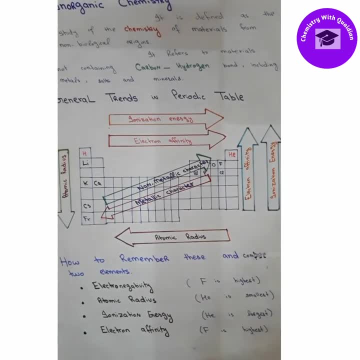 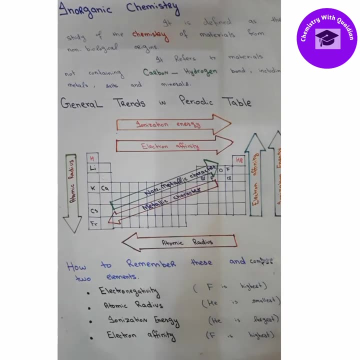 Ionization energy increases from left to right in the periodic table. Electron affinity increases from left to right in the periodic table. There are some exceptions, but these exceptions mostly lie in lanthanide, actinide, 3D series, etc. But the general concept about the trend is this. 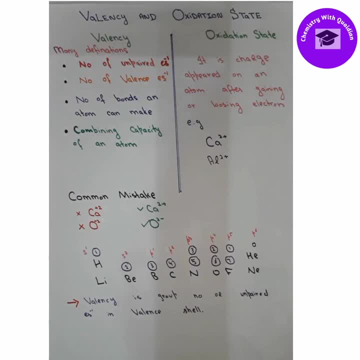 Let's talk another concept in inorganic chemistry that is very confusing. These two terms are valency and oxidation state. These are two totally different terms in the inorganic chemistry that are considered same, But these are two totally different. Let's talk about valency first. 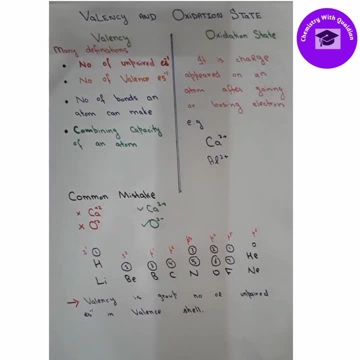 What is valency? Valency is the number of unpaired electrons, number of valence electron, number of bonds an atom can make. combining capacity of an atom. Valency is basically the group number or the unpaired electron in the valence stream. 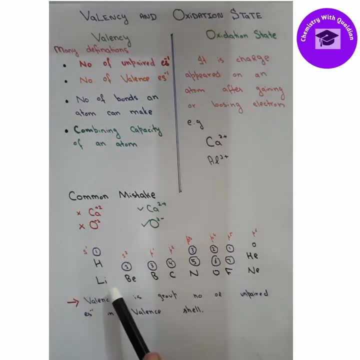 For example, If we consider hydrogen and lithium, the group 1 elements, they have one electron in the outermost shell, so their valency is 1.. Beryllium has 2 electrons, Nee has 3, Carbon has 4 electrons in the alimentous shell. So 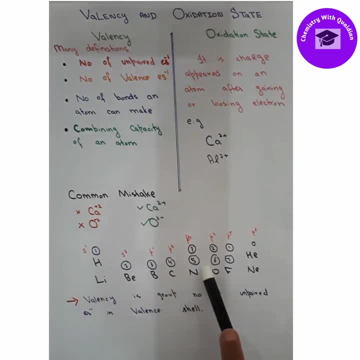 Their valency is 4.. Nitrogen has group number 5, so it's valency is 5. Also, it has 3 electrons in the outermost shell, so it's valency is also 3.. Same case with Oxygen: 6 refers to group number 3 and 6 refers to valency of group number 3.. 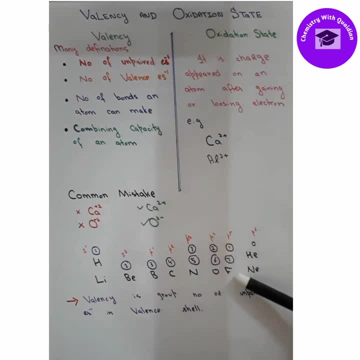 Same case with Oxygen. 6 refers to group number 3 and 2 refers to valency of group number 3.. to outermost electron: Fluorine also has one electron in the outermost shell, so its valency is 1 and also the group number is 7, so its valency is 1 and 7. both. Remember that valency has no. 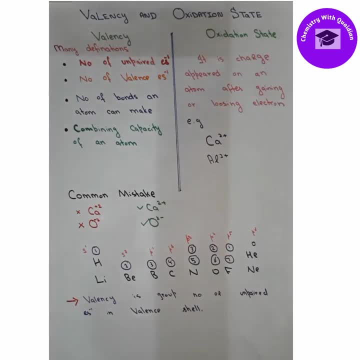 positive and negative sign. It has only a number, No negative and positive sign. And what is oxidation state? Oxidation state is the charge appeared on an atom after gaining or losing electron. For example, calcium, alkaline group metal, It has 2 electron in the outermost shell. 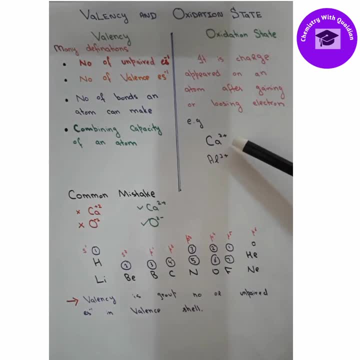 If it loses its electron, it will form a cation with 2 positive charge on it. Similarly, aluminium can lose 3 electron and have 3 positive charge on it. The common mistake that the people do in writing these symbols is that you have to put the positive sign after the number, not before.